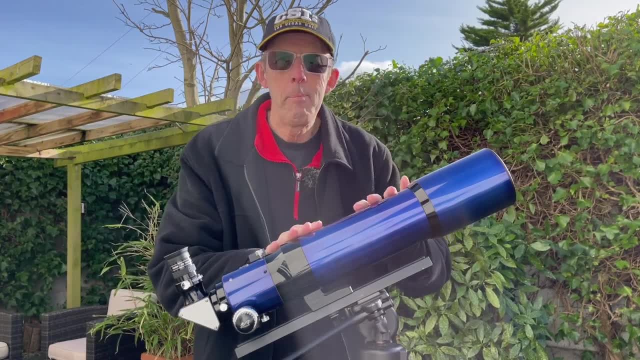 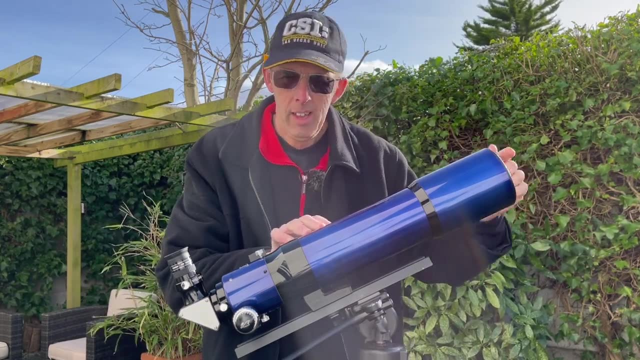 really long and and they're really really long and they're really really long and they're really quite stubby. This is kind of like a medium size refractor telescope. It has an 80 millimeter aperture on the end and it has a focal length of about 550 millimeters. 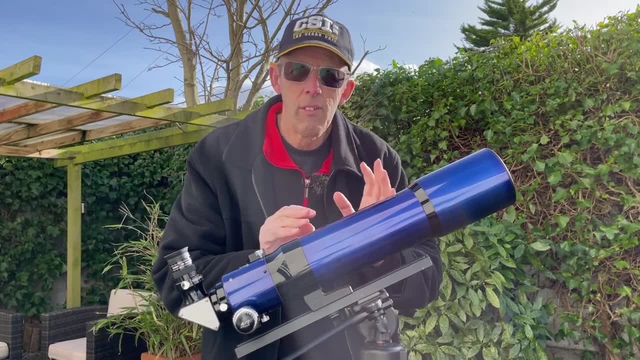 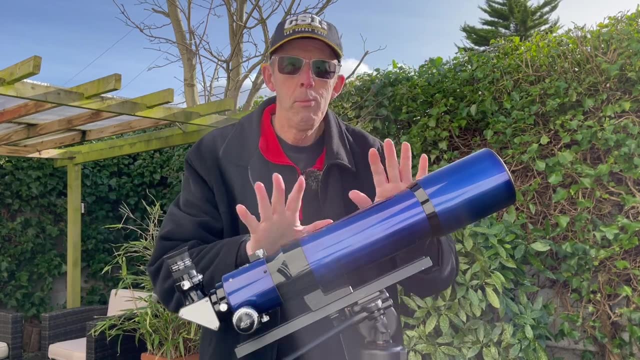 So in general terms it's fairly short focal length, but astronomy terms, The bigger telescopes tend to use mirrors and things like that to get much longer focal length. So this is more of like the sort of thing that you would use to look at large objects like the Orion nebula. 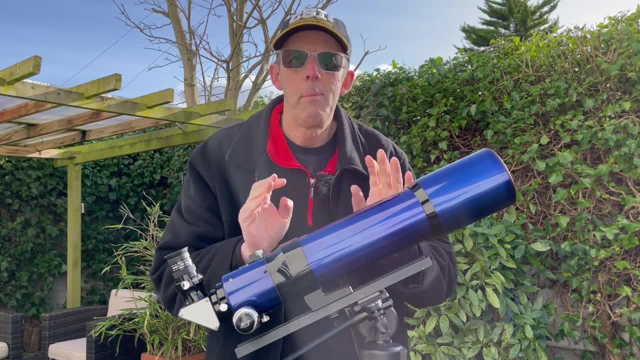 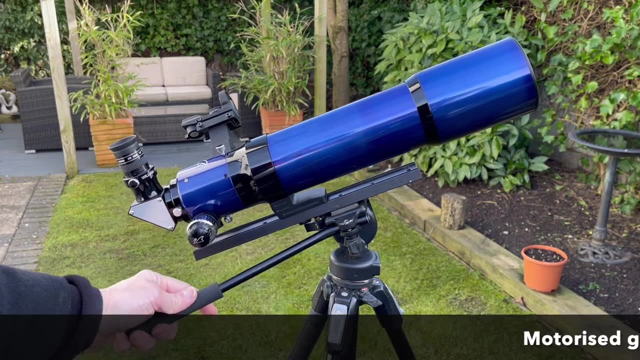 Or the moon or something like that, and they're absolutely perfect for putting your camera on. Okay, so let's take a closer look at the telescope and you can see I've got it on a bog standard camera tripod with a pan and tilt, and this is how you'd normally use. 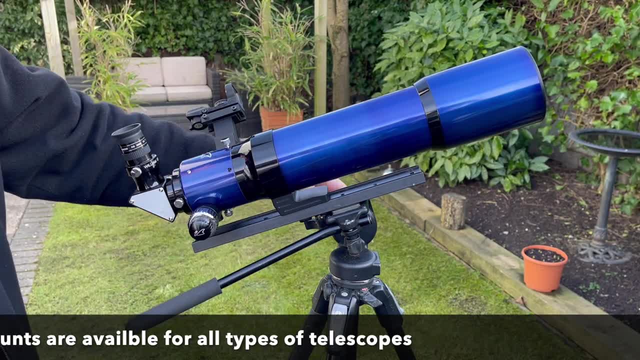 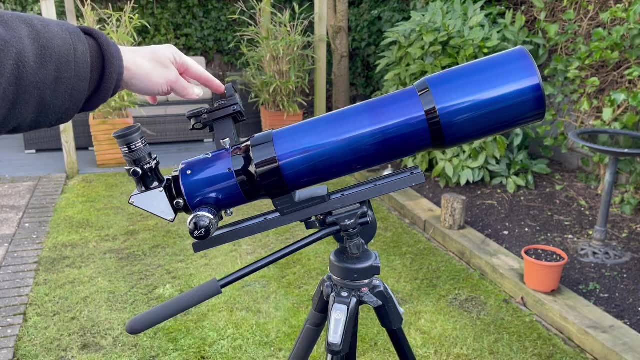 one of these telescopes, because they're a very short focal length and you basically just point them where you want them to, And I've just stuck the finder on it as well. this is what you use to point towards the object in the sky. There's a red dot in there and that helps you to find. 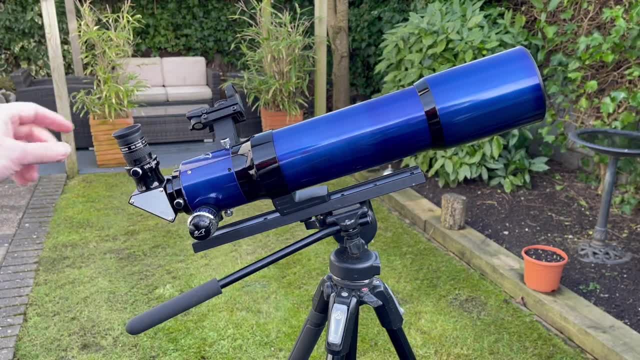 what you're looking for. So this is a very short focal length telescope and you can just point it to the object in the sky. There's a red dot in there and that helps you to find what you're looking for inside the eyepiece, because sometimes it can be a struggle to find stuff. It's an 80 millimeter. 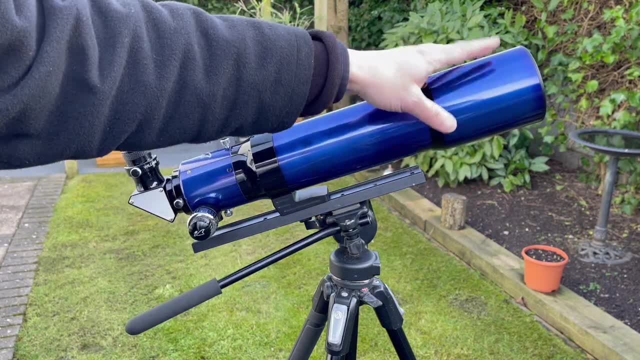 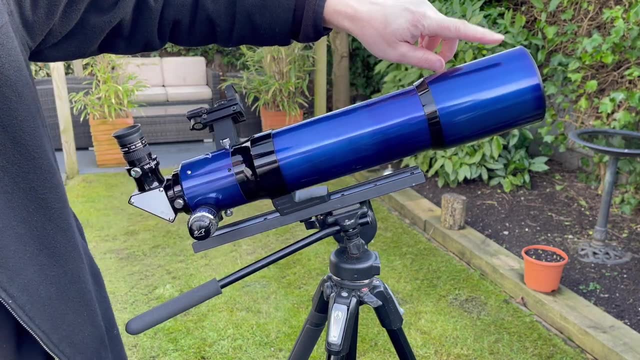 telescope, which means it has an 80 millimeter aperture at the front, or about three inches, something like that. This is also a lens hood which retracts, like that, and that helps to stop the lens fogging up if it's ever quite dewy out And coming back here you can see we've got like a. 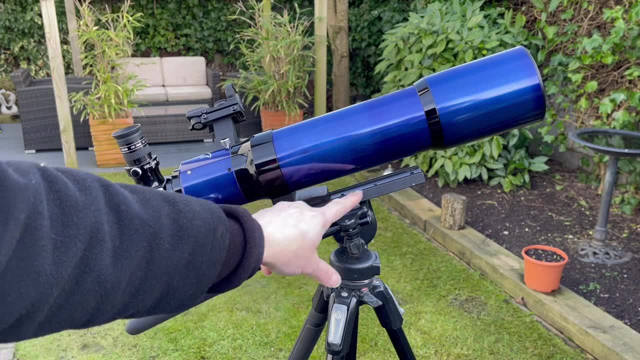 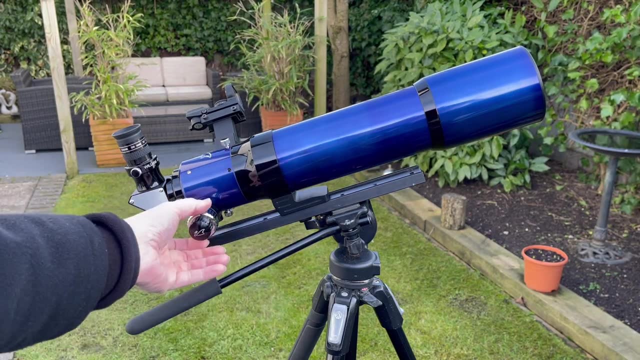 tripod foot that's like a standard tripod foot for a camera. I've had to put this bar on it as well so that it fits on my telescope mount. This is the focuser here, so when you turn this knob here, there's another one on the other side And can you see how the thing comes out there. 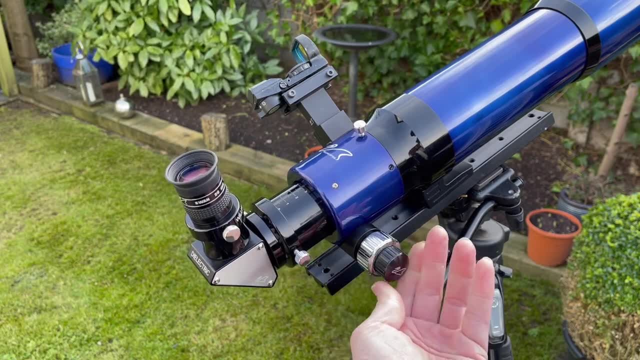 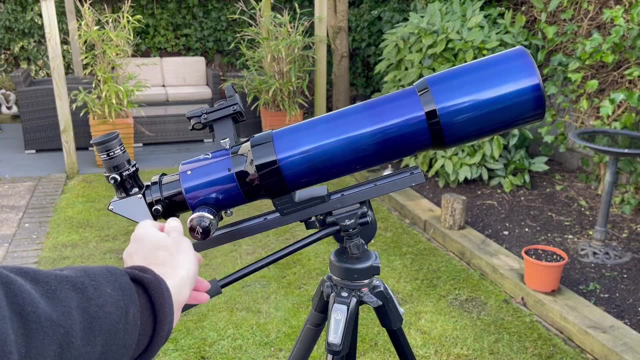 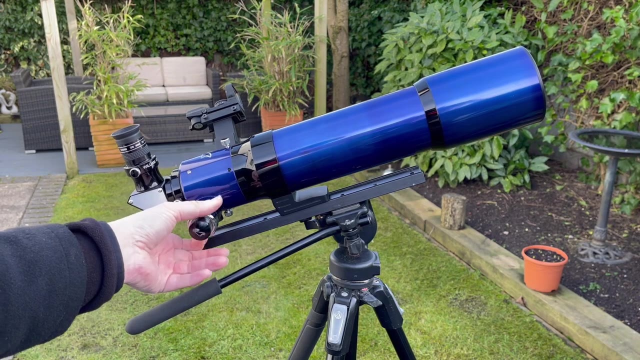 And that's how you focus the telescope. and this little one here is a fine-tuned focuser. So when you get close to focusing with that one, you can then use this one to fine-tune your focus, and then it won't jump around like it does do with the big one. And on the end, here we've got the lens hood. 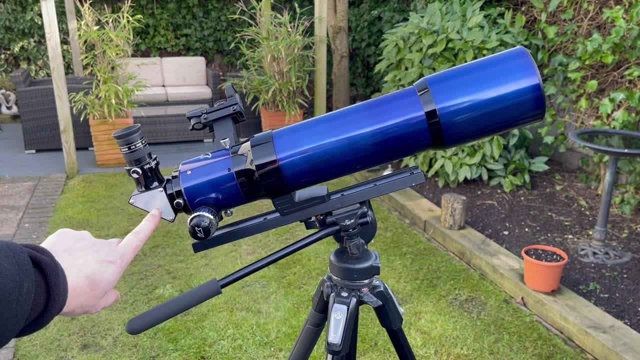 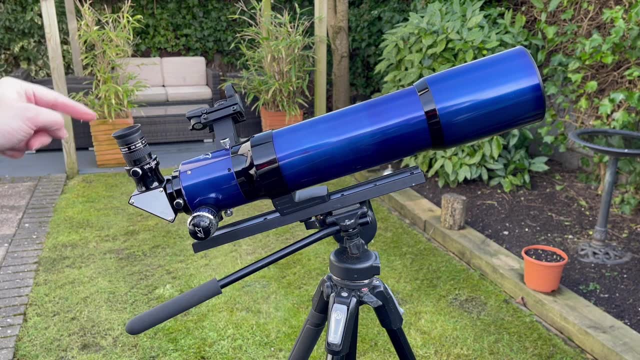 got this thing here, which is a 90 degree star diagonal. this basically means that you can look through the eyepiece at a easier angle. you don't have to strain yourself by looking straight through. like that. you can also get a 45 degree angle, fine, so you look through it like that instead. so there's. 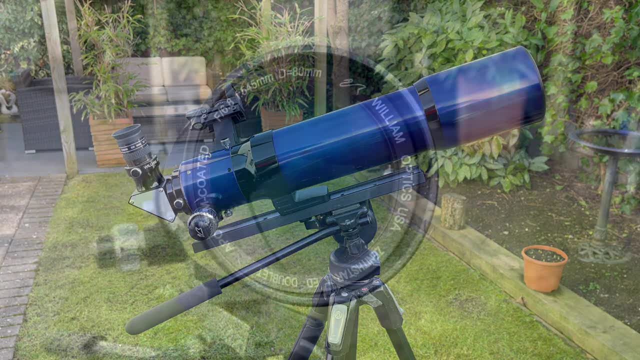 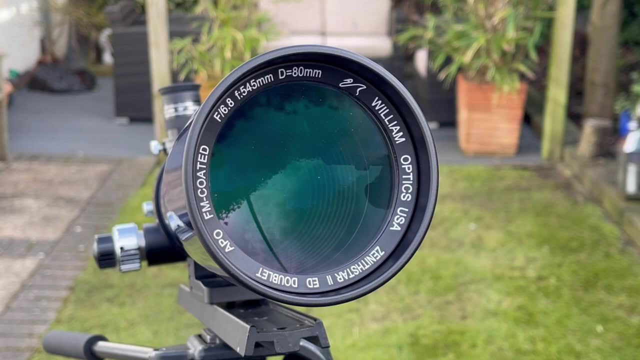 a, there's different ways in which you can look through the telescope. okay, so we're now looking at the front of the telescope and i just thought i'd mention what all these words and numbers mean, because it does look really, really confusing. well, it's fairly simple to point out that it's made by 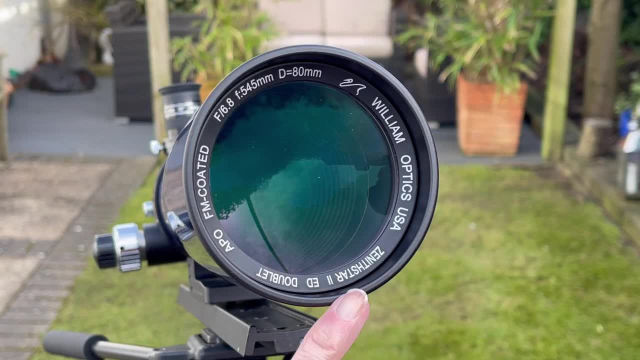 william optics of the usa and the model number is a zenith star 2 ed, which stands for extra dispersion. this is something that you might see on a telephoto camera lens. if you have one and double it, well, that's another thing as well, because these telescopes, they come with different lens groupings. 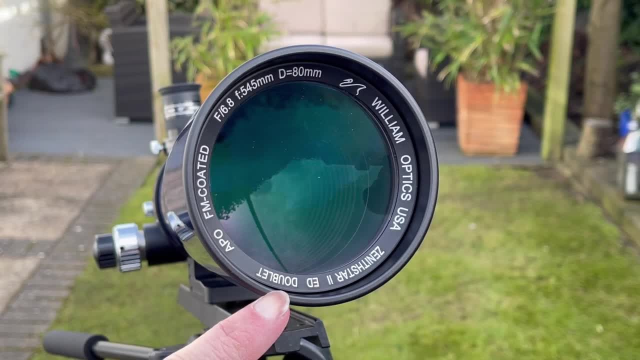 the cheapest ones only have a single lens grouping and they're called acromats. this is known as an, and this has a double lens group grouping. now most apochromatic tend to be triplets and they have three lens groupings and they're more expensive. but william optics have managed to make an apochromatic out of a. 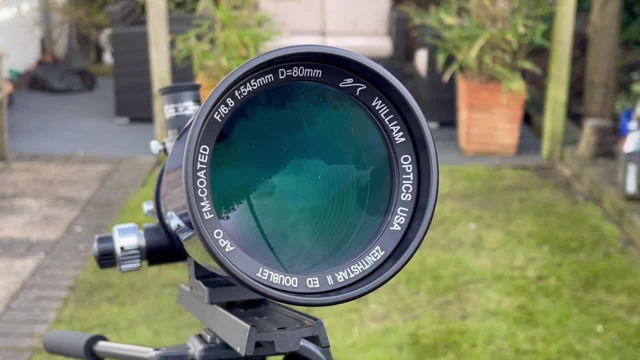 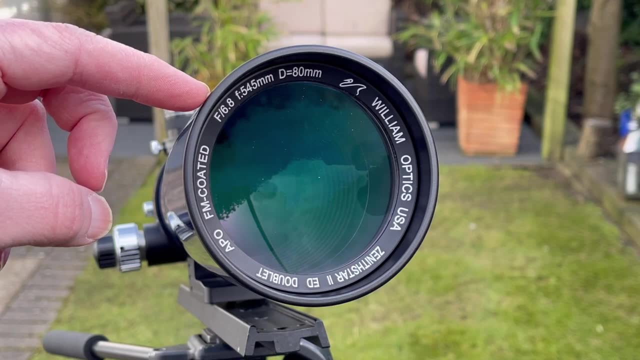 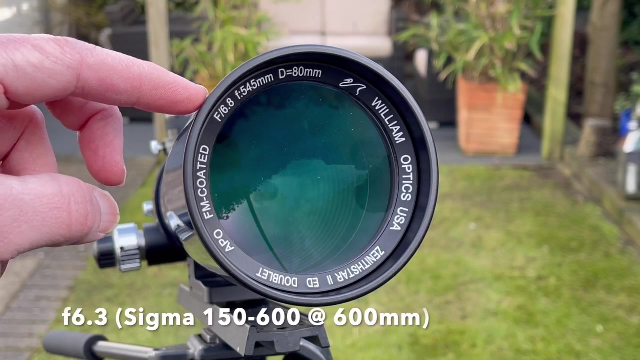 doublet in this particular telescope just coming around here. we have an aperture here of f 6.8. now if you've got one of those long telescope lenses like the sigma- 150 to 600 is it, you might notice- go up to something like 6.8 when you're at 600 mil. so that's very similar to the- uh, the same thing. 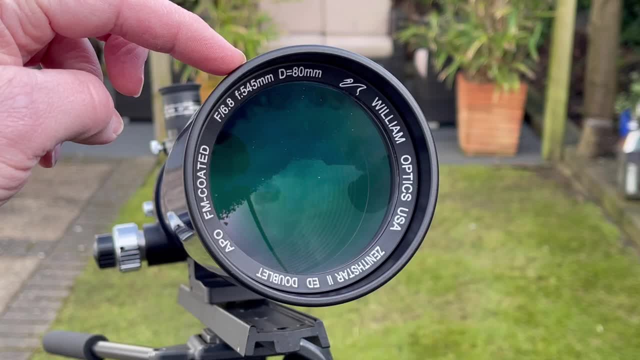 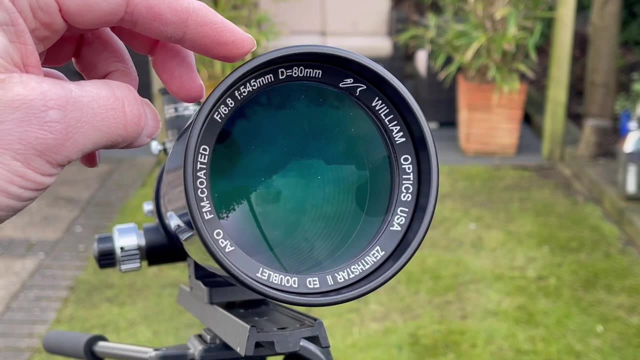 that you would get on a camera lens and, as you can see here, we've got a focal length. this is a focal length- 545 millimeters, which- astronomy terms- telescopes- is fairly short. we're fairly wide field with this, with this telescope, and that's why i think it's a great starter scope, because we're 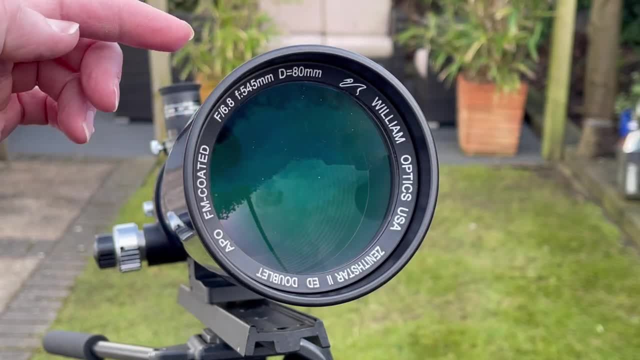 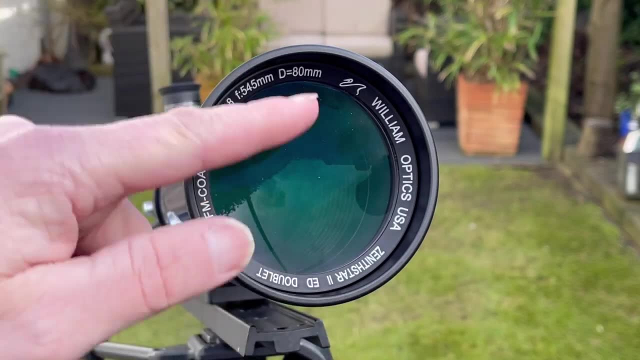 not getting too close to stuff. we want to start wide if we can, and up here we've got 80 millimeters the width. this is the width of the objective lens. okay, so, as you can see, i've got an eyepiece on the end of this telescope. 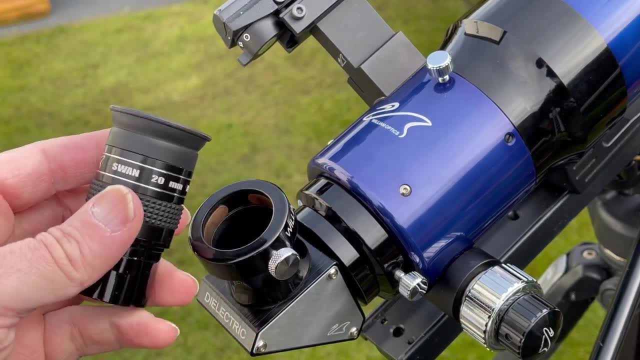 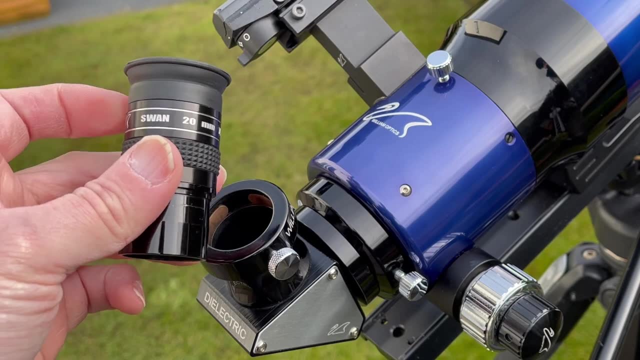 and this is a 20 millimeter eyepiece, which is a fairly wide field eyepiece for a telescope. now i'm going to tell you how you can find out how much this will magnify the object you're looking at. so say, you're looking at the moon and you've got a 20 millimeter eyepiece. 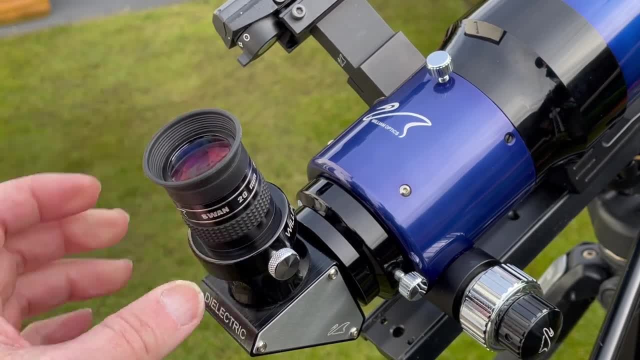 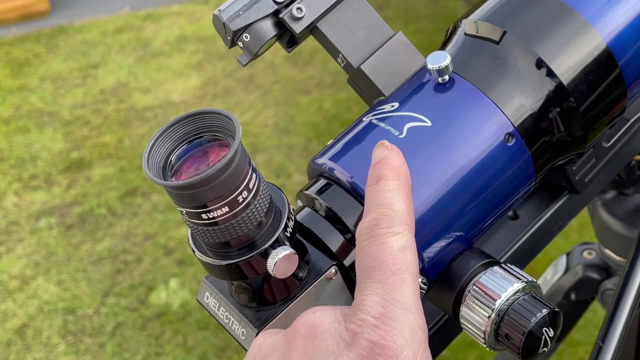 on this telescope, i can tell you that it will magnify the moon 27 times, and the reason for that? the telescope is 540 millimeters roughly. i've rounded it off to 540 millimeters now. 20 goes into 540 27 times and that's how you get a magnification of 27 times. 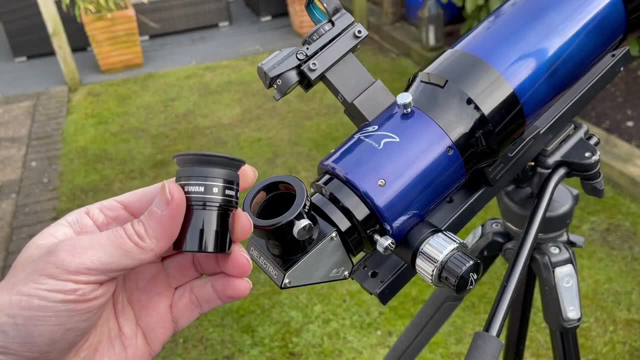 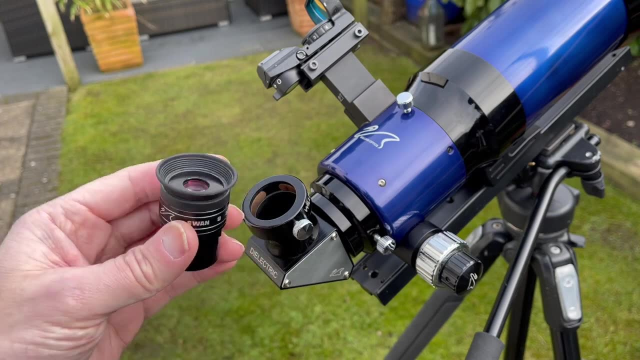 using a 20 millimeter eyepiece. okay, so i've now got this other eyepiece and this is a nine millimeter eyepiece, but let's pretend it's a 10 millimeter, just to make it easier to to do the calculations. you can see there that the aperture on the eyepiece is a bit narrower than on the 20 millimeter eyepiece. 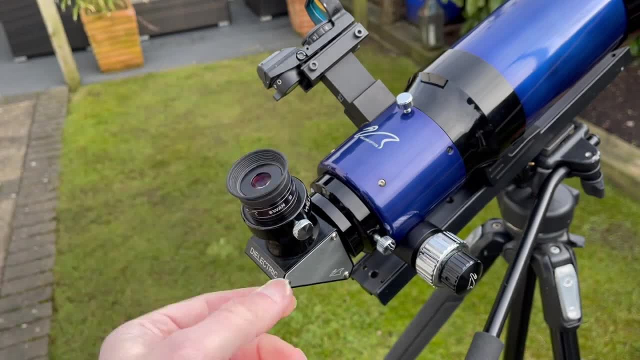 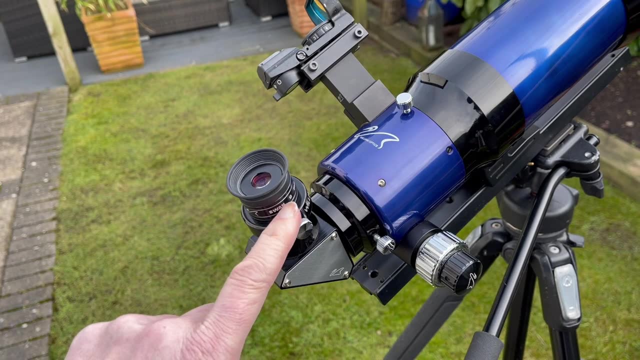 so if i put that in there now, what will happen is that will magnify the moon 54 times, because if this is a 10 millimeter eyepiece, it goes into the focal length of this telescope 54 times, because it's a 540 millimeter telescope, the smaller the number on the eyepiece, the more 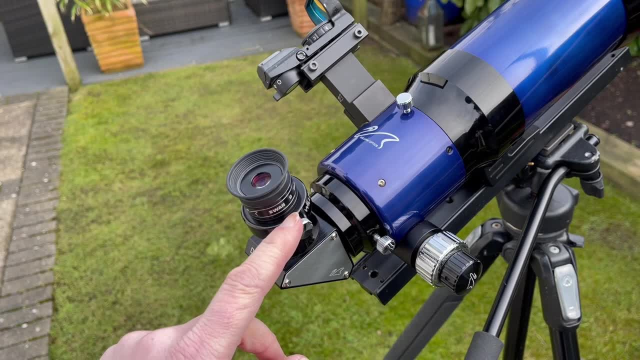 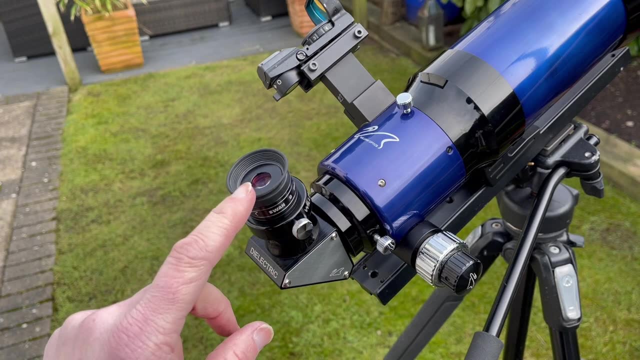 powerful it will be, but at the same time you have to be careful that you don't use too small an eyepiece, too powerful, or too small an eyepiece because it will magnify the moon 54 times that the subject becomes a little bit too dark, because the subject will be darker. 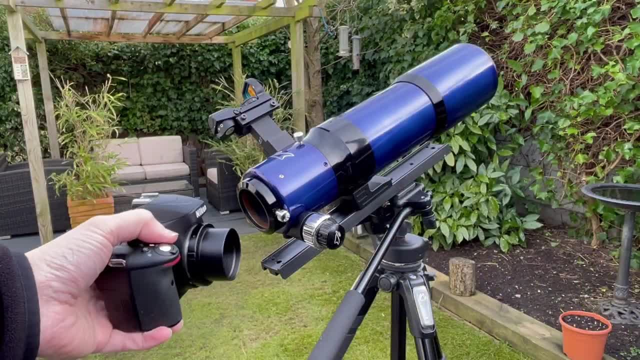 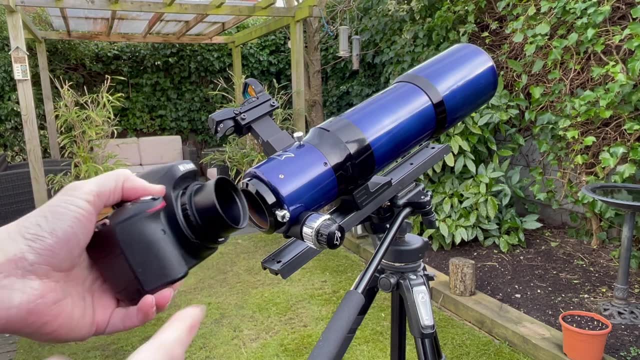 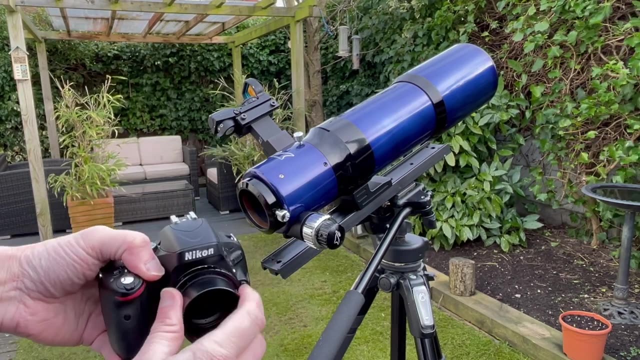 when you're using a smaller eyepiece. and now, if you're interested in putting the camera on, like, i've got this nikon d5100 camera here which is a getting on a bit now. but you can see here i've got this thing on on it here in place of a lens and this is called a t adapter and and ring. 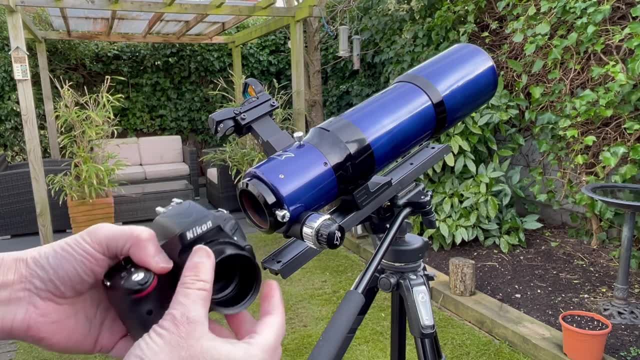 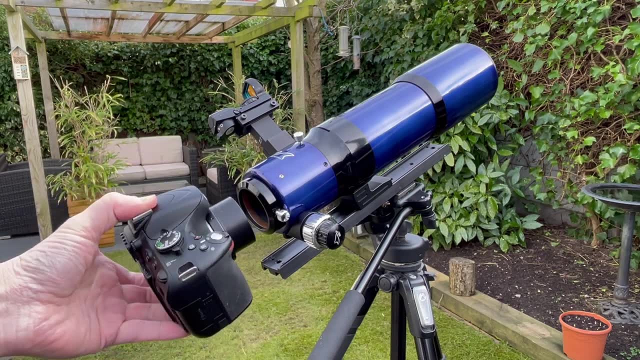 and you can see here this allows. they're not expensive. they're only about 15 or 20 pounds. um. you can get them on on ebay or whatever and basically that allows you to put the camera. i've taken the thing off for the eyepiece there as. 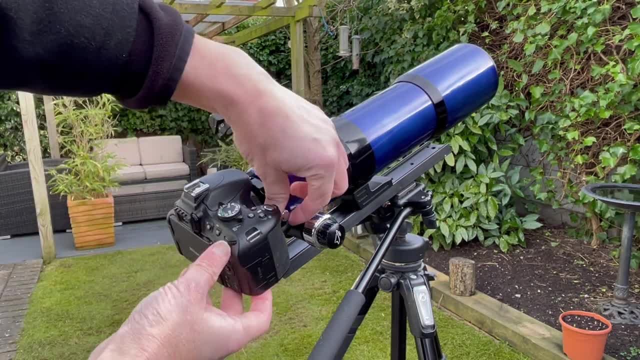 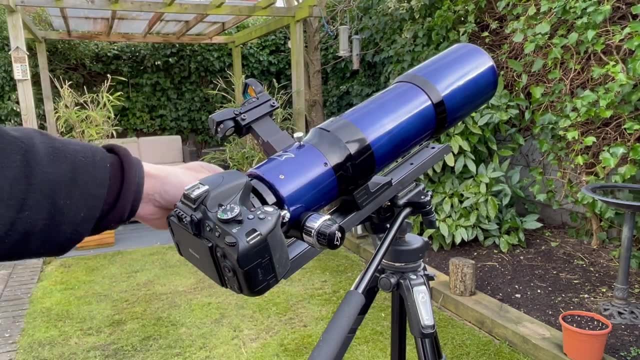 you can see, and it simply just slots into there like that, and that's all you have to do. and then you're ready then to point the camera up to the moon or or whatever, and remember that you use these to focus. you haven't got an auto focus, so you have to use these things here and that's.